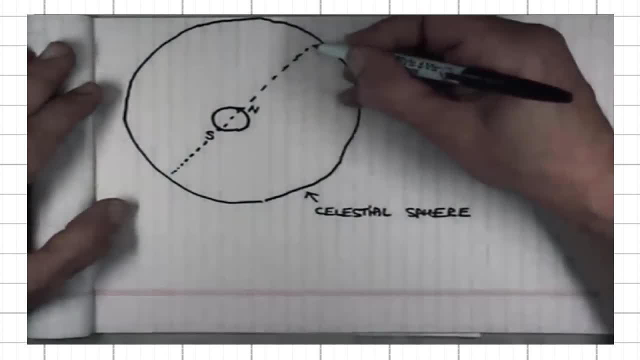 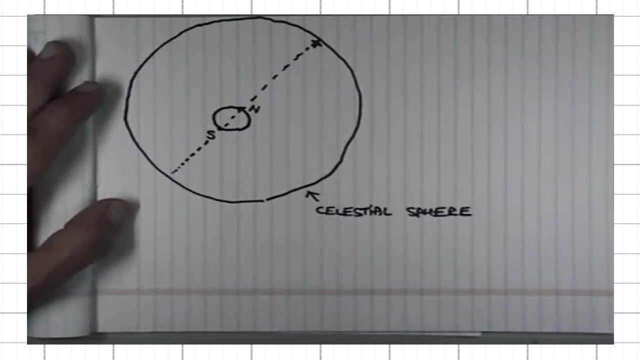 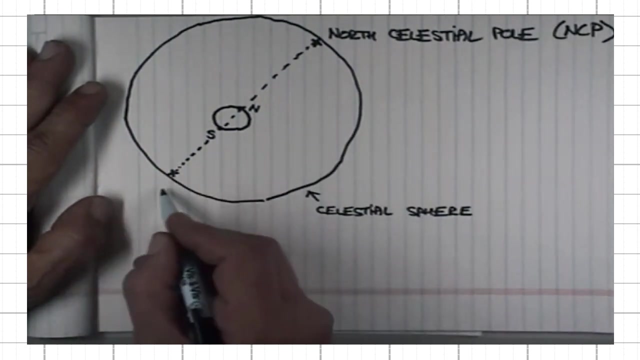 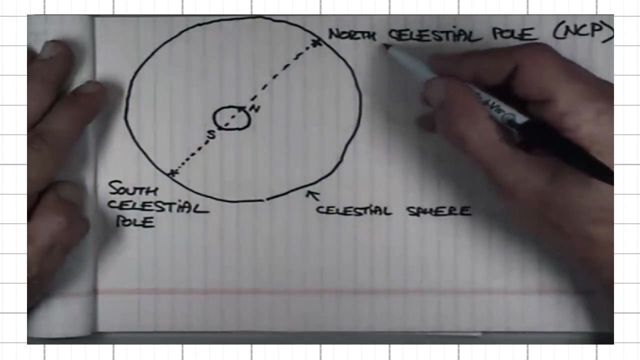 all the way out to the celestial sphere. it would puncture it at two points: One that is directly above the Earth's North Pole and it's called North Celestial Pole, or NCP, in short. The one that is directly above the South Pole is called South Celestial Pole. 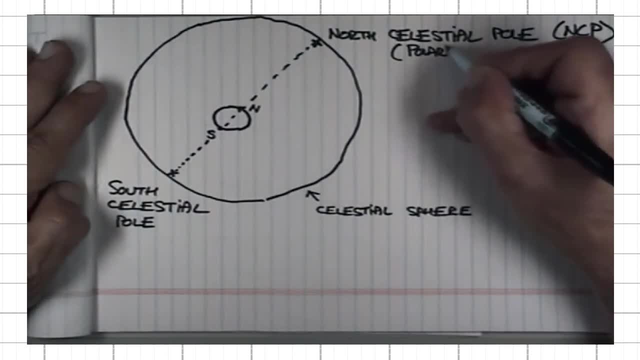 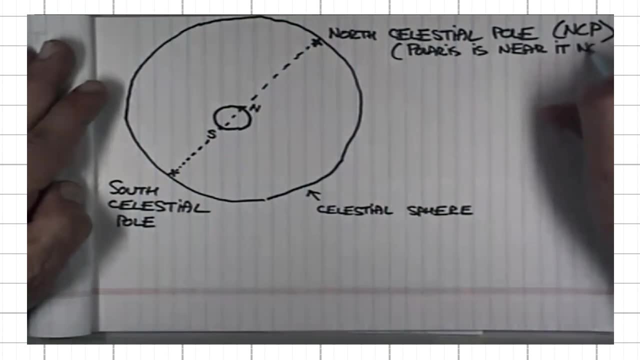 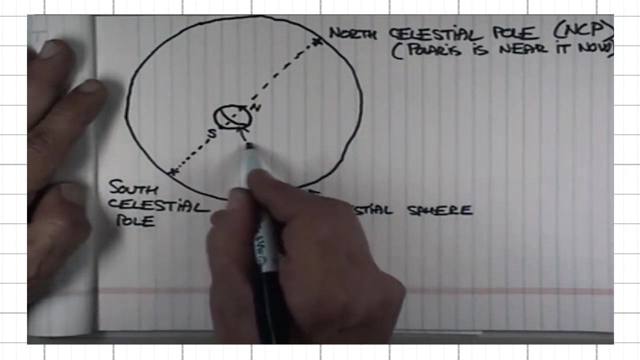 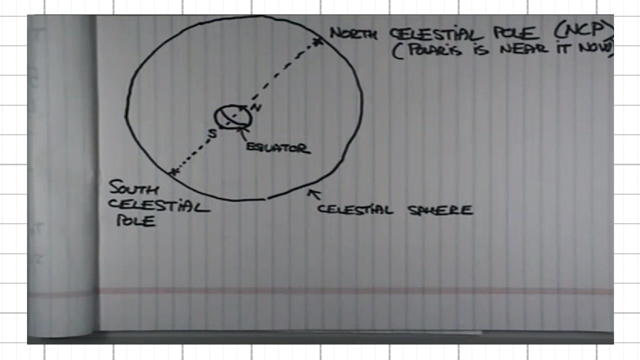 As I mentioned before, Polaris, NCP is near it now and no star close to the South Celestial Pole. These are the two important points on the celestial sphere. Then here is the Earth's equator and the line on the celestial sphere that is directly. above the Earth's equator is what we call celestial equator. Here is the Earth's equator. Here is the Earth's equator. Here is the Earth's equator. Ok, Then, for an observer that is at mid-latitudes North, like us say here, this would be the. 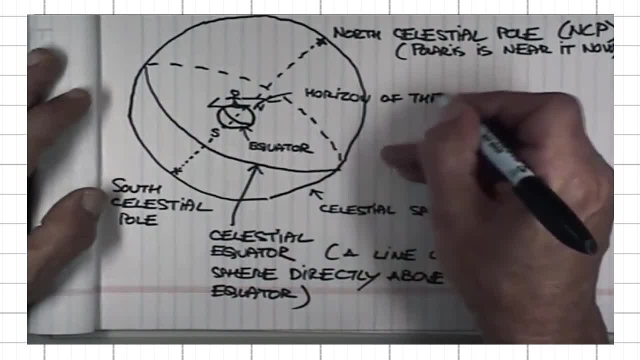 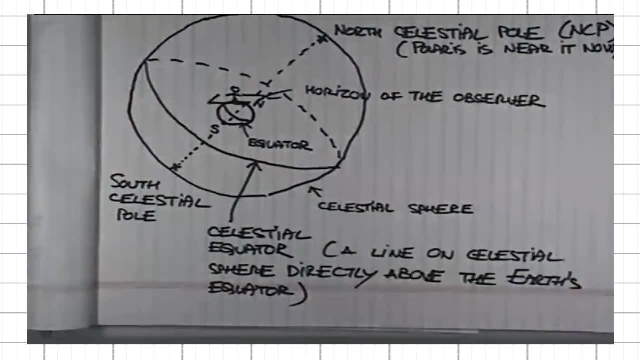 observer's horizon. This would be the observer's horizon. Remember I mentioned that last time when we discussed how Aristotle deduced that we must be living on the sphere. When one travels south, one starts seeing new stars above your horizon, at your current location. 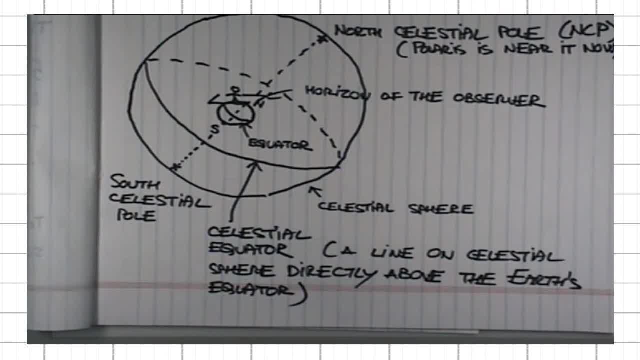 You can see things that are above your horizon and you can't see anything below your horizon. Observer can see everything that is above the horizon and nothing that is below his horizon. As a result, what you see depends on where you are on the Earth, because 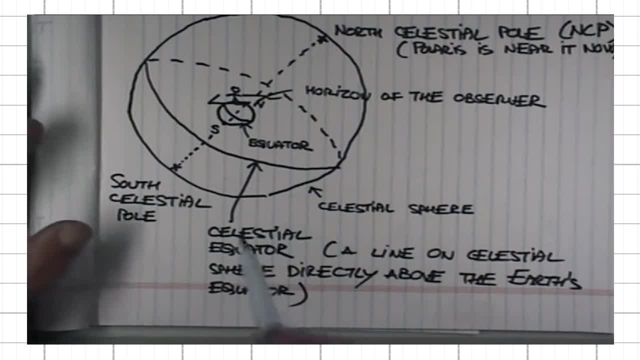 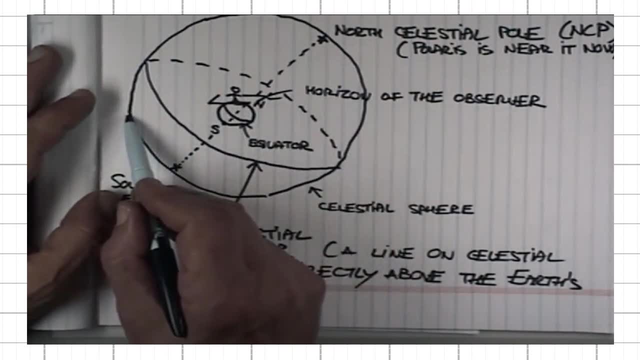 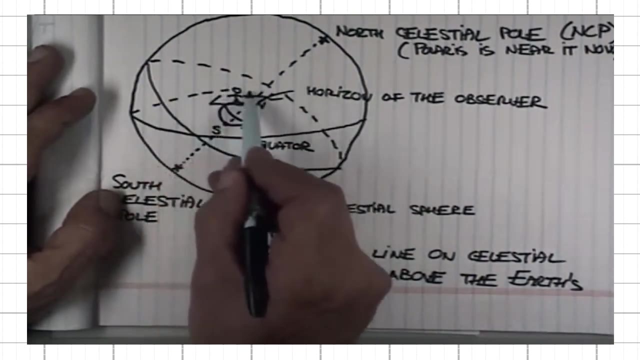 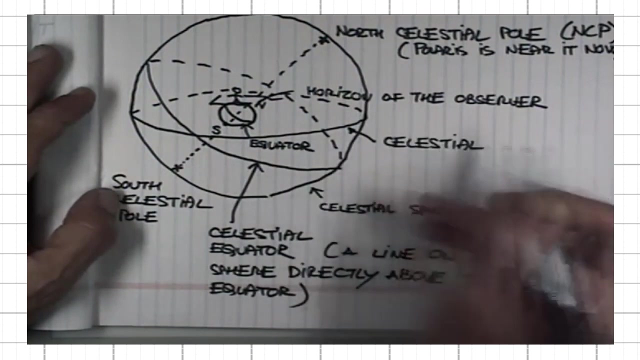 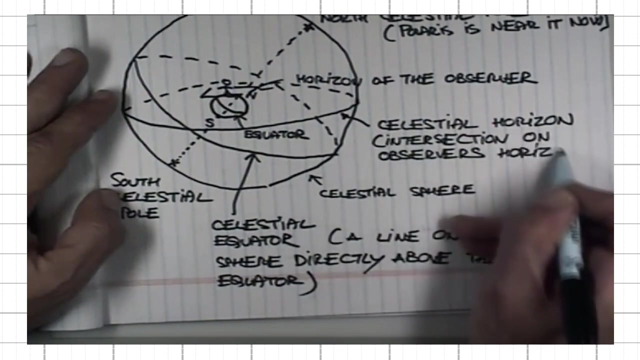 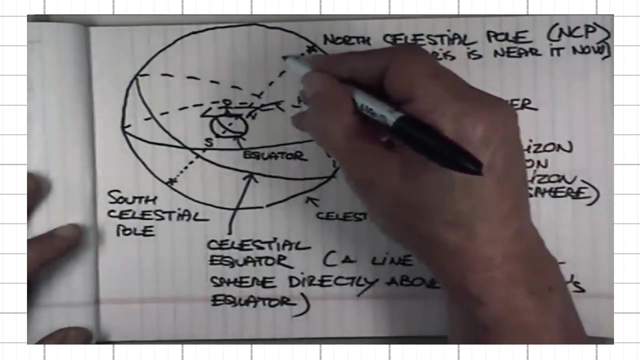 that determines the location of your horizon. If I would extend the plane of the horizon all the way out to the celestial sphere, it would make a line on the celestial sphere that we call celestial horizon, Because the Earth is spinning from west to east. it's not going to move.